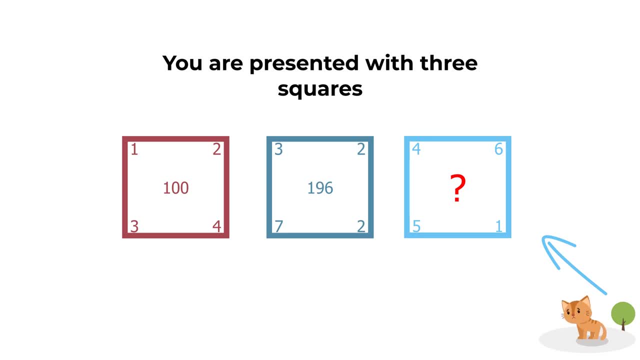 square has numbers four, six, one and five in the corners And number in the middle in the square is missing. You have four different choices to calculate missing number: Choice A 244,, choice B 250,, choice C 256, and choice D 262.. Do you see the answer? Give yourself 10 to 15. 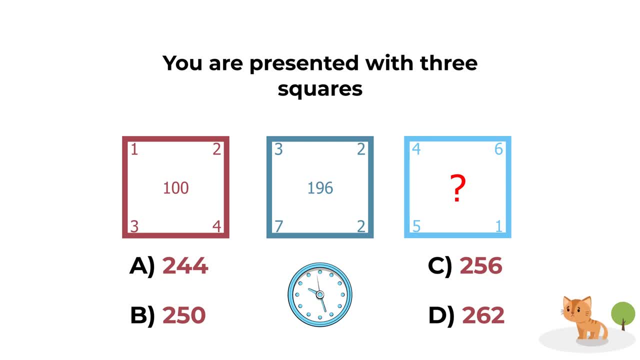 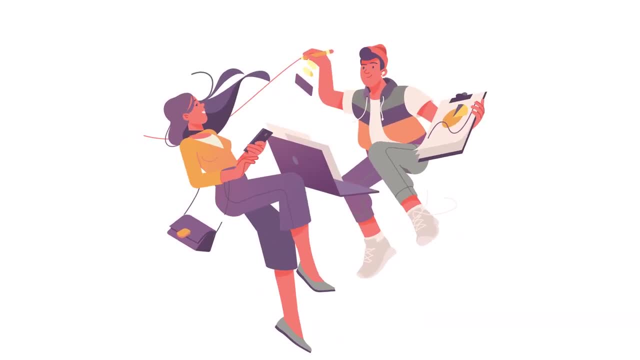 seconds, maybe 20 to 30 seconds, by pausing this video and trying to calculate the missing number. Did you figure it out? Let's go ahead and move forward so we can get to the correct solution together. As you can see, the number is missing. So let's go ahead and move forward so we can get to the 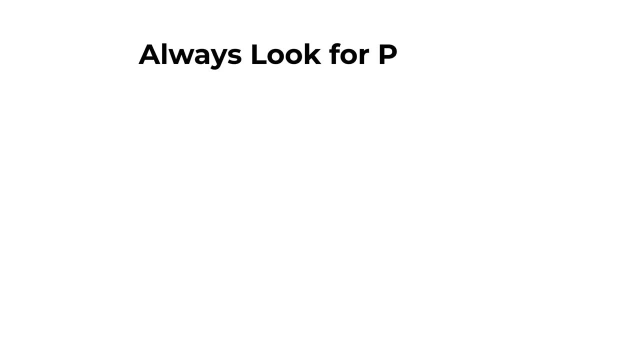 correct solution together. As you can see, the number is missing. So let's go ahead and move forward so we can get to the correct solution together. As usual, to solve any challenge. my advice to you always look for patterns And then the pattern here is that the middle number. 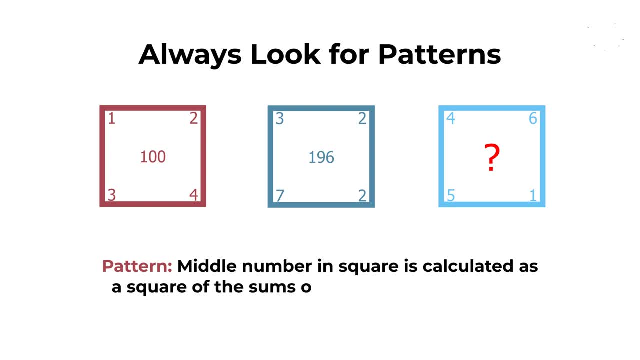 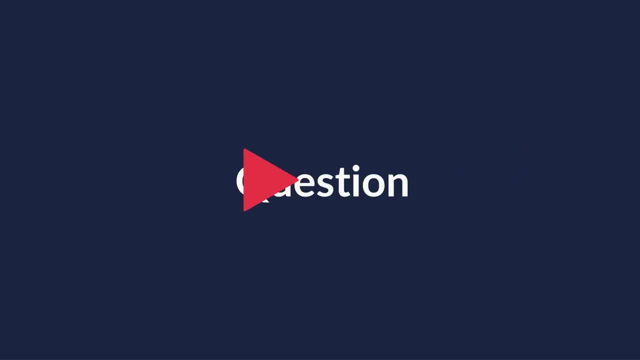 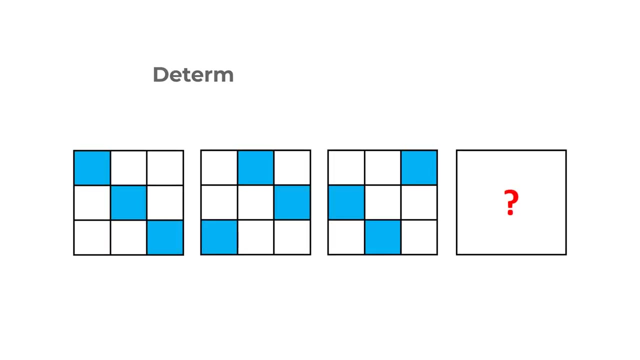 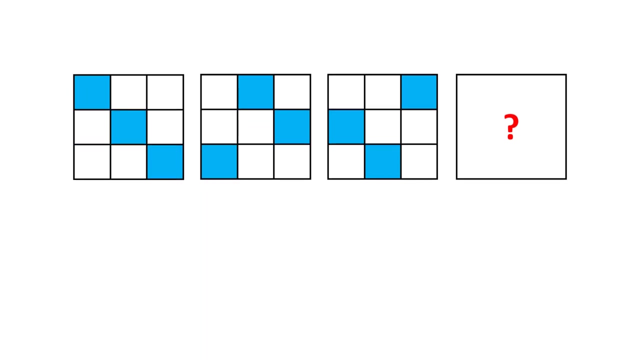 So there are problems on the test. Here is a very interesting problem that you may frequently get on the test. You need to determine the next equation. in your system. You are presented with the sequence of large squares. Each large square contains 9 small squares inside. 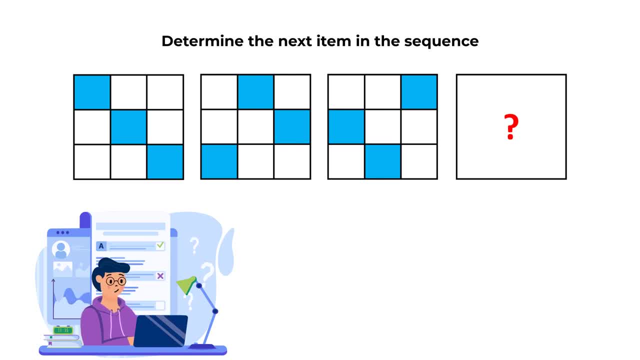 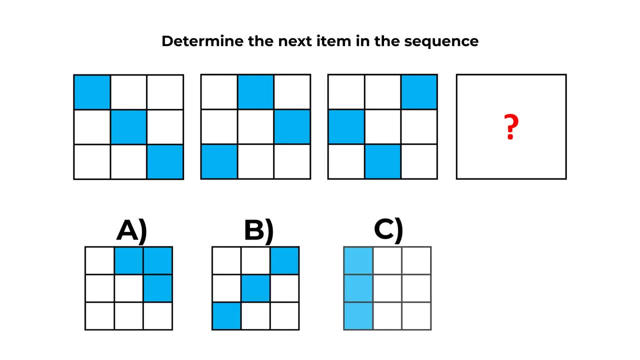 And each square is of a different color. You need to determine the next equation in the sequence and you have four different choices: Choices A, B, C and D. Do you see the answer? Give yourself 10 to 15 seconds. 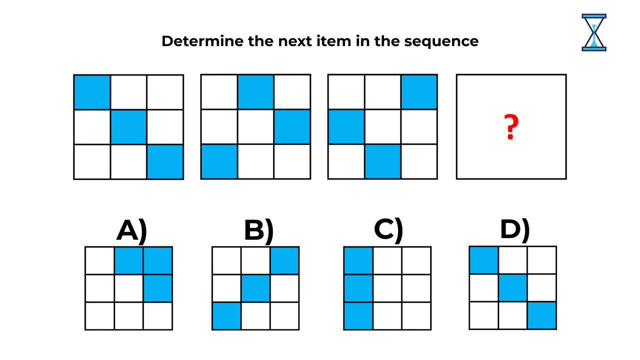 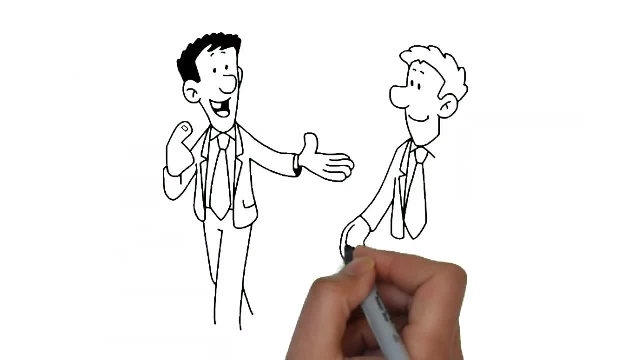 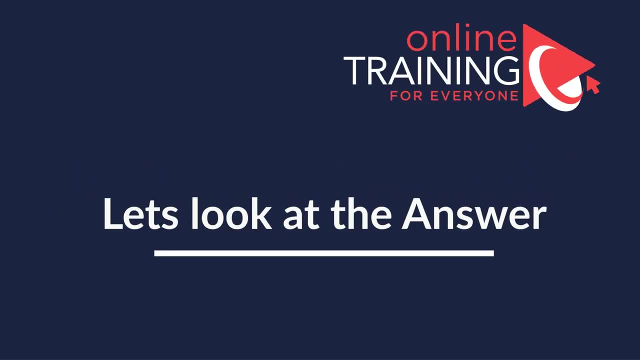 maybe longer, maybe 20 to 30 seconds, to see if you can come up with the solution. Did you figure it out? Let's go ahead, move forward to get to the correct solution together. As always, my advice to you is to look for patterns. 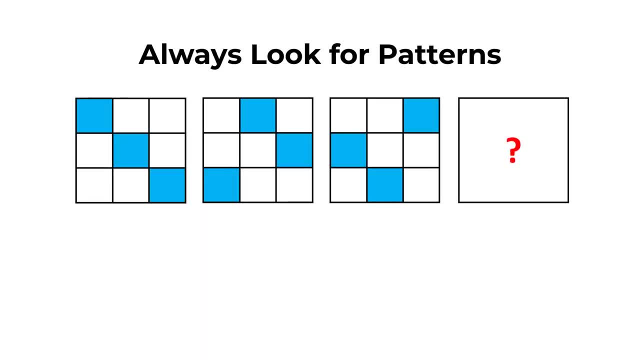 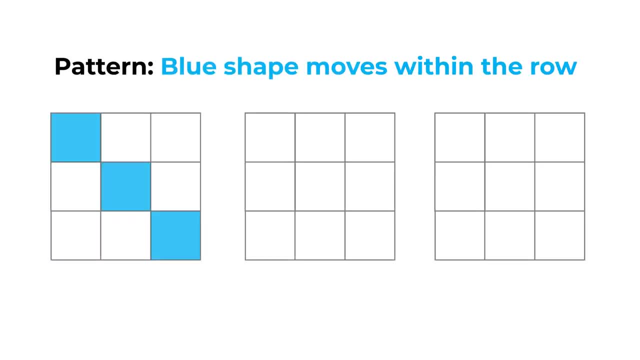 And determining the pattern is key to solving this particular problem. What you need to know to answer this particular question is that the blue shape moves within the row of the larger shape. In each row, the blue shape moves from left to right one step at a time. 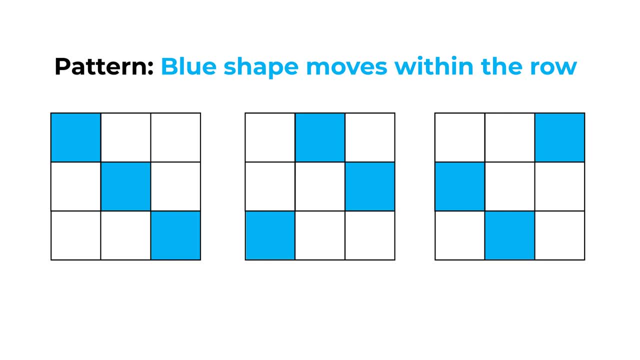 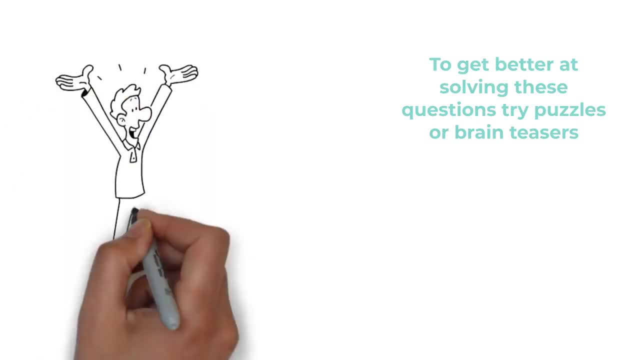 And once the blue shape reaches the end of the row on the right, it reappears on the left. So the correct answer here is choice D. Hopefully you've nailed this question and now know how to answer similar problems on the test. 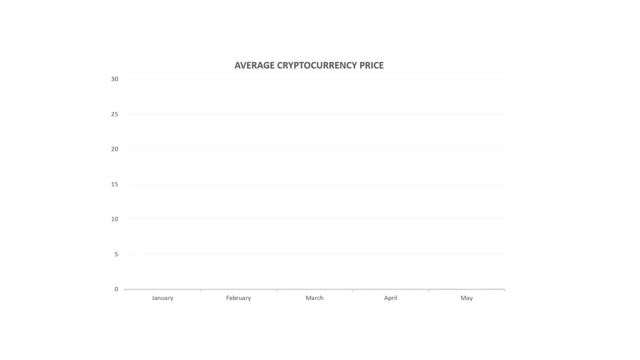 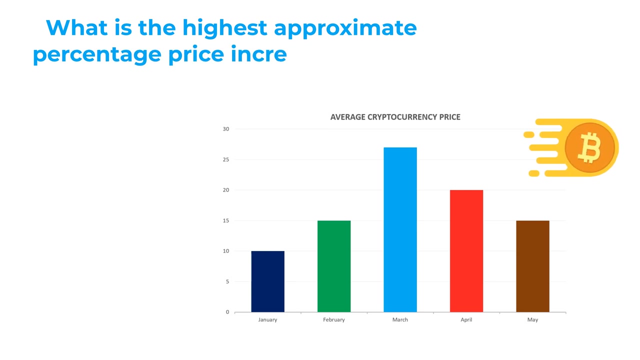 And now here's the practice problem for you. You're presented with the chart that shows the average price of cryptocurrency, And this chart shows the average price for each month from January to May. You need to calculate what is the highest approximate percentage price increase. 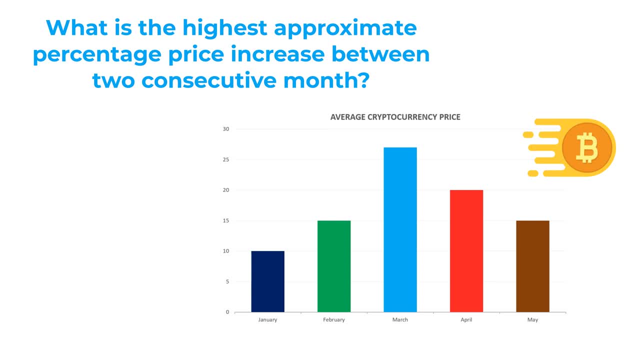 between two consecutive months And you're presented with four different choices: Choice A- 60%, Choice B- 70%, Choice C- 80% And choice D- 90%. If you know the answer, please make sure to post it in the comment section of this video. 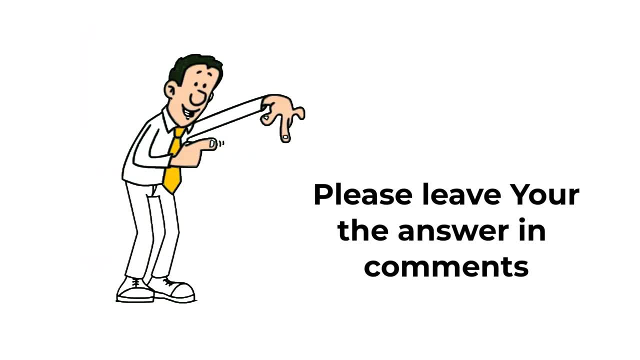 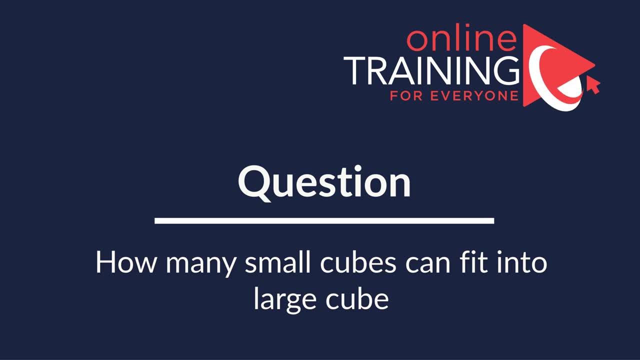 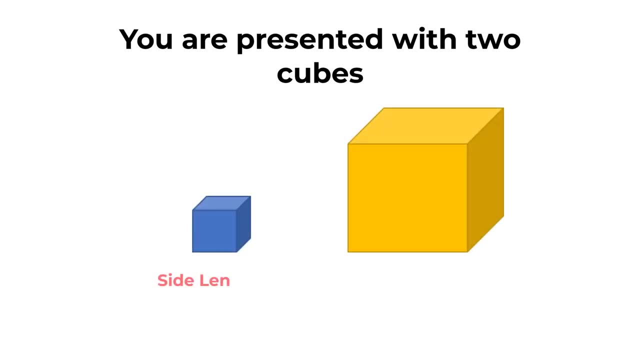 so I can give you the feedback. Thanks for participating and good luck. Here's a cool question which you frequently see on the chat. You're presented with two cubes. One cube has side length equal one unit, And second cube is a larger cube. 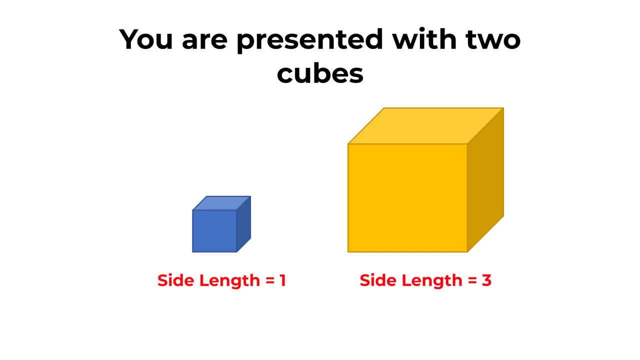 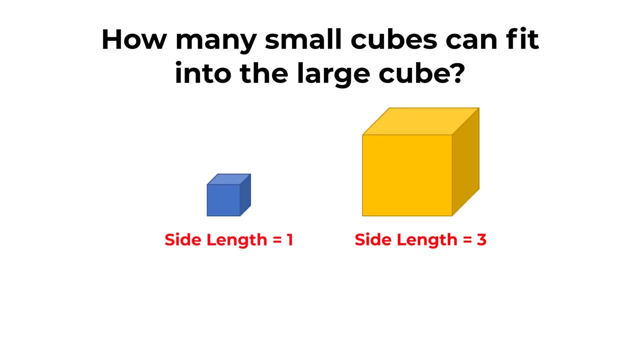 and it has side length equals three units. So the question is how many small cubes can fit into the large cube? And you have four different choices: Choice A, 9. Choice B: 18. Choice C: 27. And choice D: 81.. 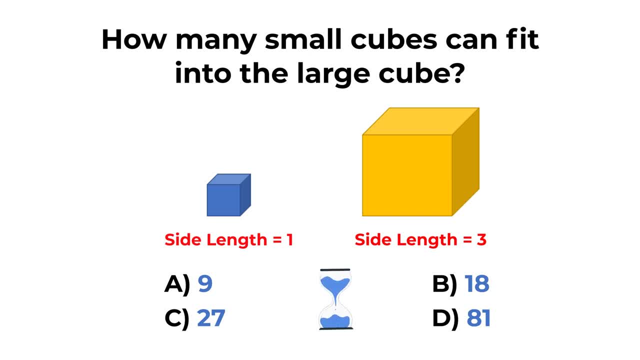 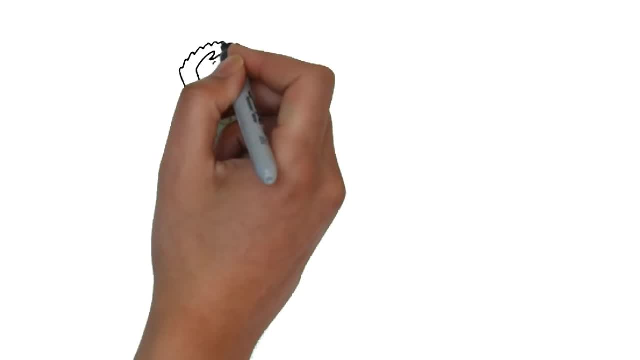 Do you know the answer? Give yourself a few moments to calculate it. Maybe 20 to 30 seconds. This is about as much time as you get in the real test, Ready or not. let's go ahead and get to the correct solution together. 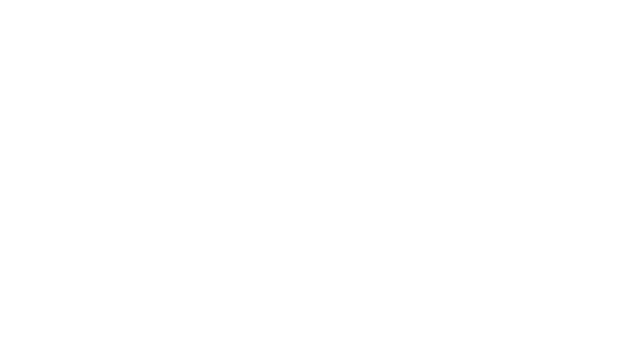 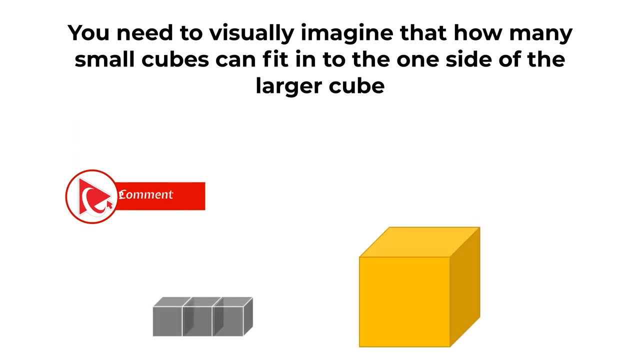 To solve this challenge, you need to visually imagine how many small cubes can fit into one side of the larger cube. And the answer is that three small cubes can fit on each side of the large cube. And since cubes are always larger, Since cube is 3-dimensional, the number of small cubes that can fit into the large cube 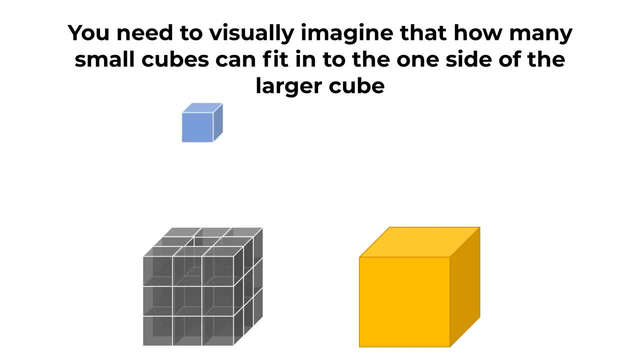 can be calculated using the formula: 3 multiplied by 3, multiplied by 3, which is equal 3 cube- that's where the word cube might be coming from- which equals 27.. Since cube is 3-dimensional, the number of small cubes that can fit into the large cube- 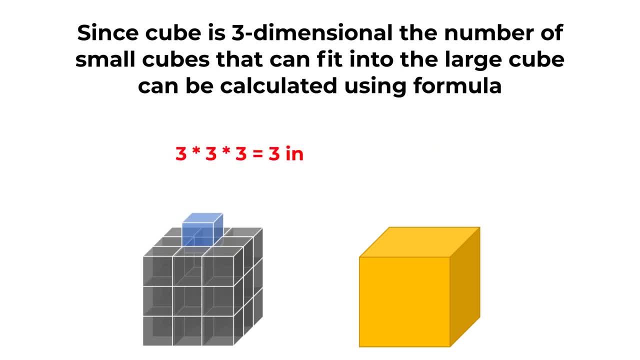 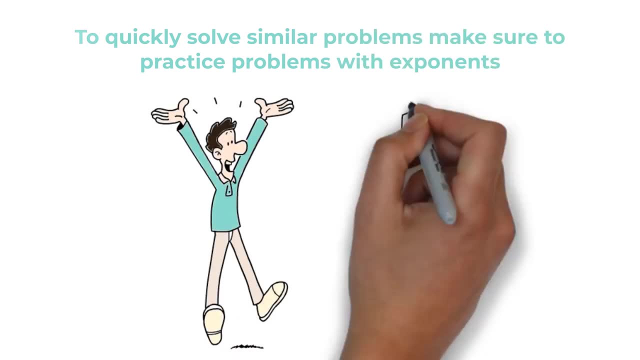 can be calculated using the formula: Remember: 3 multiplied by 3 multiplied by 3 equals 3, cube equals 27.. So the correct choice here is choice C 27.. Hopefully you've nailed this question and now know how to answer similar problems on the test. 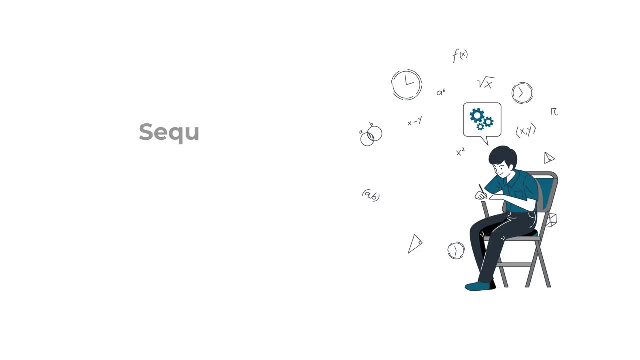 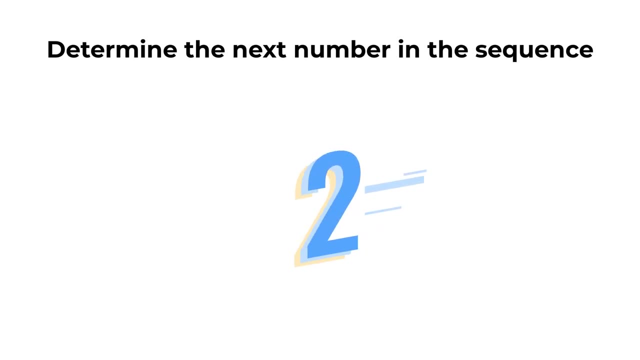 It is almost guaranteed that you will get questions like this on every test. You're presented with the sequence of numbers And you need to determine the next number in the sequence. In this case, the numbers are 2,, 10,, 30,, 68,, 130, and the next number is missing. 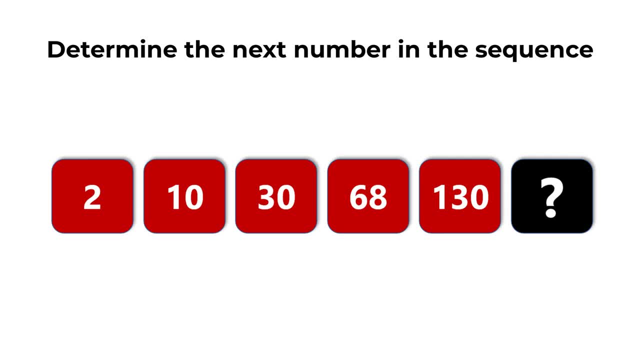 Can you determine what comes next in the sequence? You're presented with four different choices: Choice A 216.. Choice B: 218.. Choice C 220.. And choice D 218.. And choice C 222.. Now might be a good time to pause this video to see if you can come up with the answer. 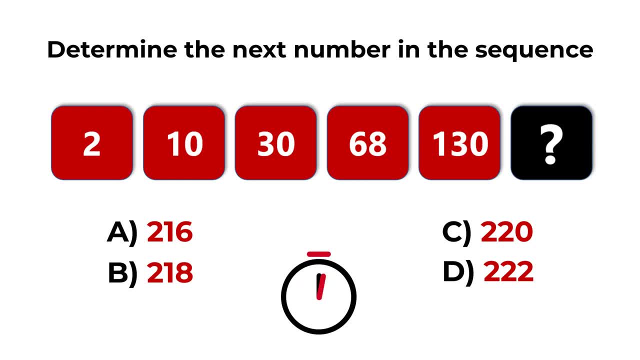 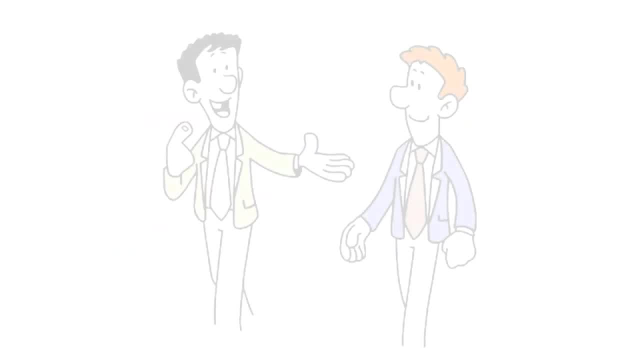 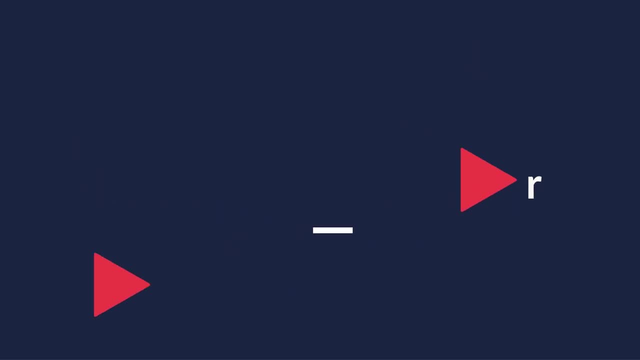 Give yourself 20 to 30 seconds. That's about as much time as you get in the real test, Ready or not. I'm moving forward so we can get to the correct solution together. When dealing with sequence questions, my recommendation to you is always look for patterns. 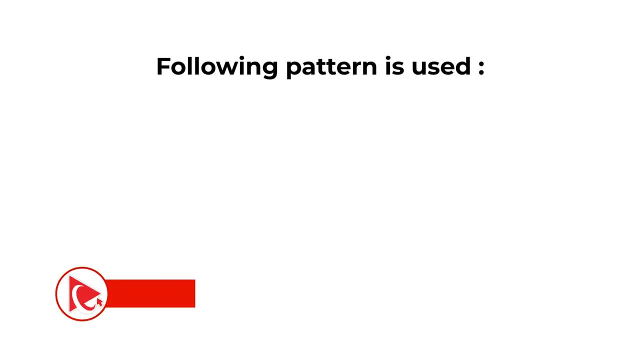 And to determine the answer. in this case, you need to look for patterns And to determine the answer in this case, you need to look for patterns And to determine the answer in this case, you need to look for patterns. In this case, we need to use the pattern n³ plus n. 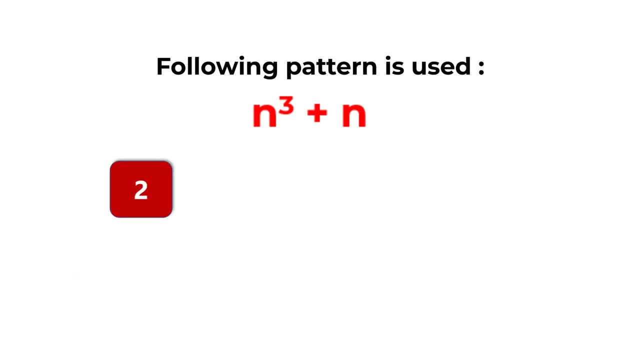 So it starts with the first number, which is equal 2, and it was calculated as: 1³ plus 1 equals 2.. Next number was calculated as 2³ plus 2 equals 10.. The following number was calculated as: 3³ plus 3 equals 30.. 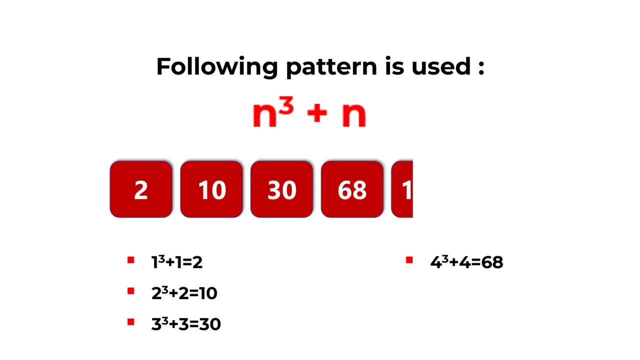 Then 4³ plus 4 equals 68.. 5³ plus 5 equals 130.. Then 4³ plus 4 equals 68.. 5³ plus 5 equals 130.. which means that the missing number should be calculated as 6 cube plus 6 and the result would: 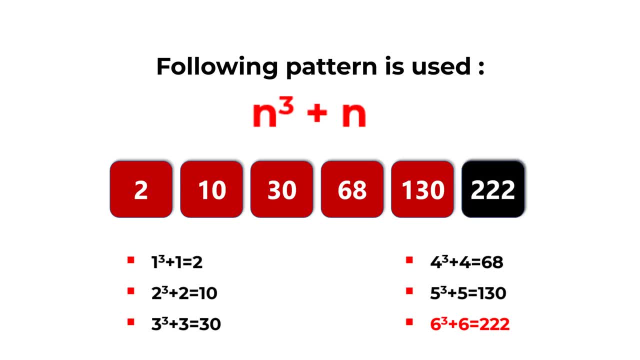 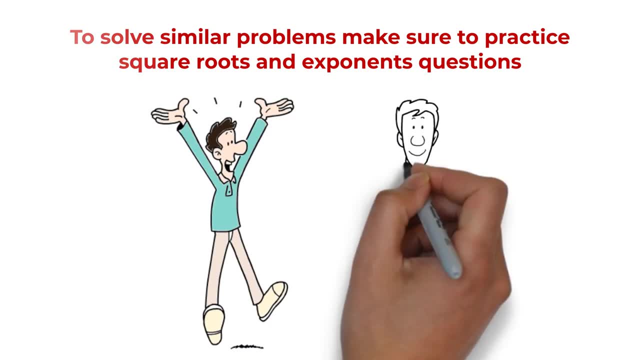 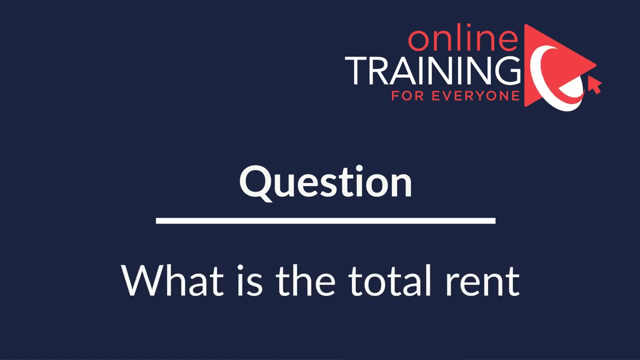 be equal 222. so the correct answer here is choice d 222. hopefully you've nailed this question on your own and now know how to answer similar problems on the test. here's an interesting question you may need to know, not just for the test, but also if you're trying to rent the house. 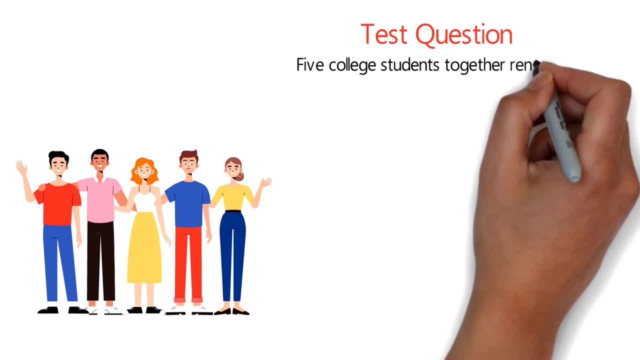 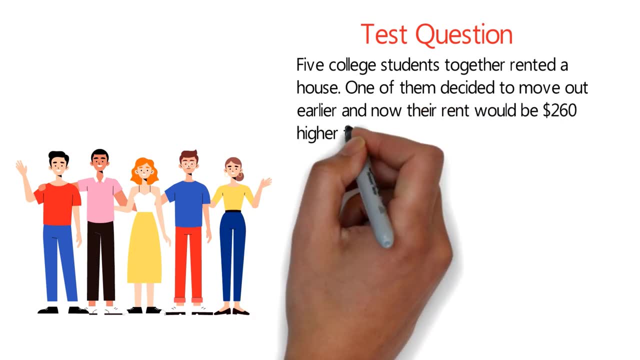 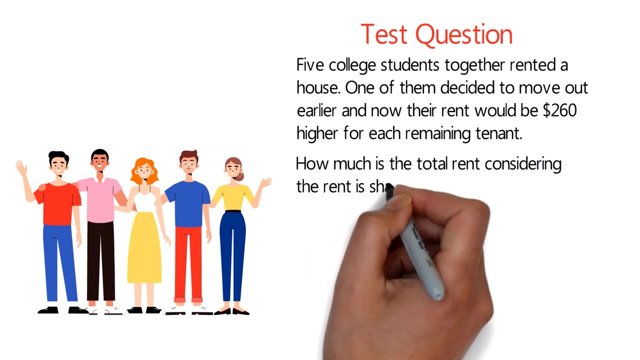 five college students together rented a house. one of them decided to move out earlier and now their rent would be 260 dollars higher for each remaining tenant. what is the cost of the total rent, considering the rent is shared equally among students, and you're presented with four different. 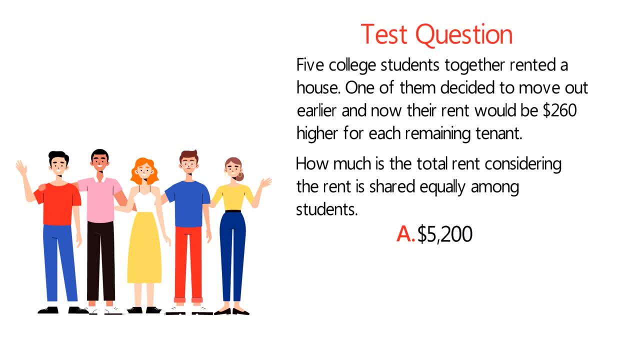 choices: choice a: you, five thousand two hundred dollars. choice b: three thousand one hundred twenty dollars. choice c: two thousand six hundred dollars. and choice d: two thousand three hundred and forty dollars. give yourself 20 to 30 seconds. maybe pause this video to see if you can come up with the answer. 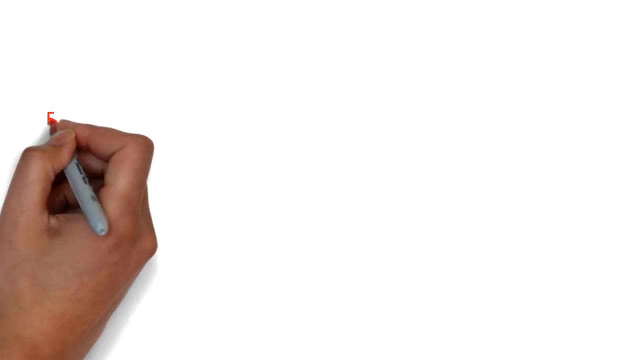 on your own. let's go ahead and solve this challenge together. one of the easiest way to solve this challenge is to create a formula. let's start by solving the following question by defining a variable, and we will define this variable as s, which would represent an initial. 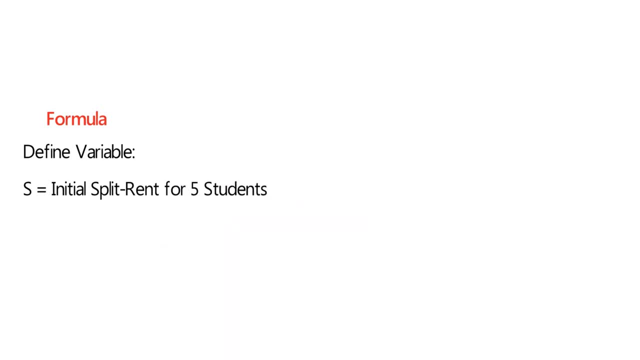 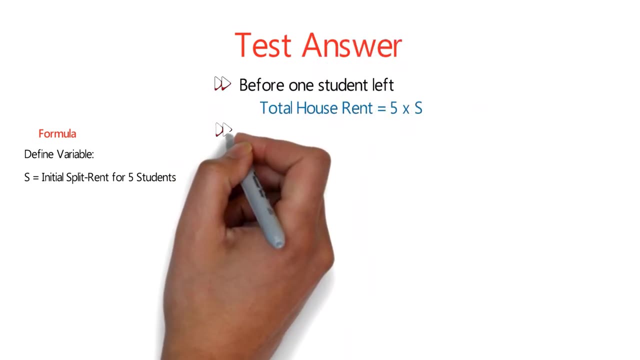 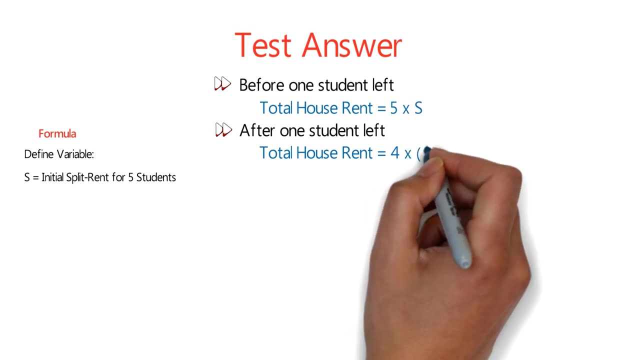 split trend for five students. so using this formula, we can calculate the total house rent as five multiplied by s, which means that after one student left, the total house rent could also be calculated as four multiplied and then the value in parentheses s plus two hundred sixty dollars. using both approaches. 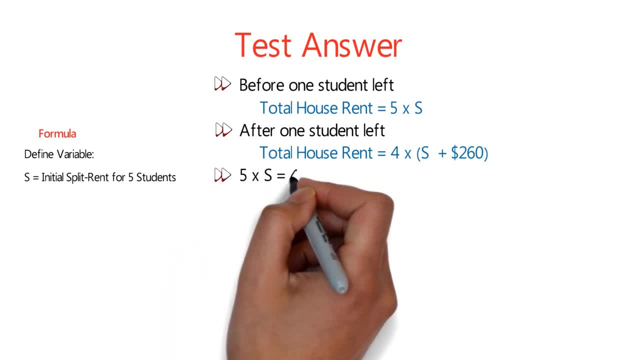 we can create an expression: five multiplied by s equals four multiplied, and then the value in parentheses, s plus two hundred sixty dollars. once we simplify it, we'll get to the equation: five s minus four s equals one thousand forty dollars, which means that the s equals one thousand forty dollars. 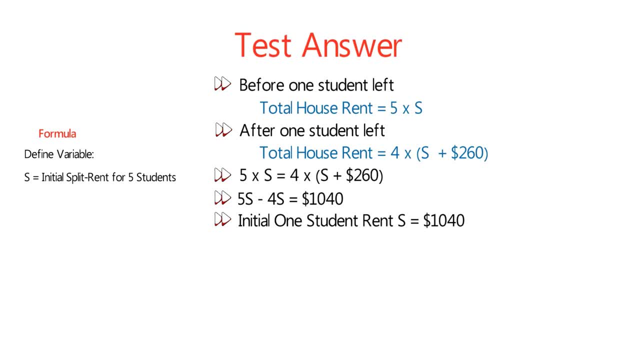 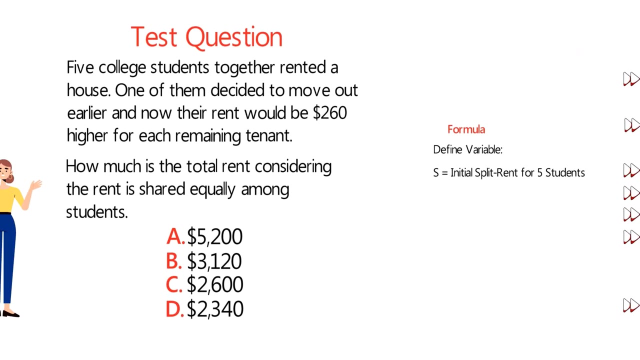 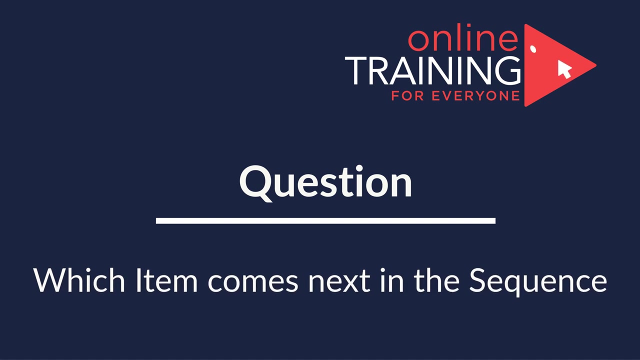 which represents initial one student trend. to calculate total house rent, we need to multiply five by one thousand forty dollars and the result will be five thousand two hundred dollars. so the answer is choice a. five thousand two hundred dollars. hopefully you've nailed this question and now know how to answer similar. here is an example of excellent problem that you frequently see. 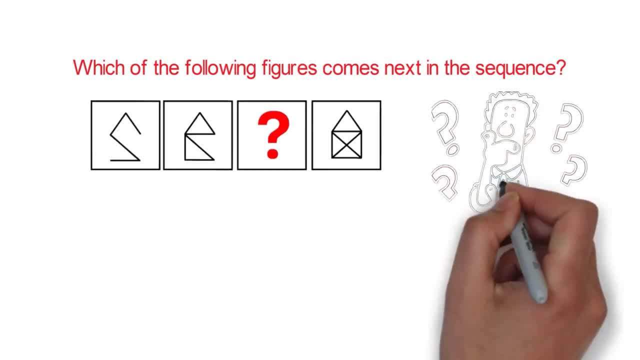 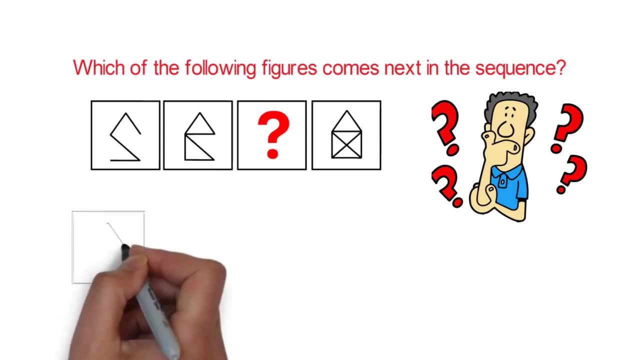 on the test. you're presented with the series of shapes and you need to determine which of the following shapes comes next in the sequence. You have choices A, B, C and D. Take a close look at this picture to see if you can come up with the answer. Give yourself 10 to 15, maybe 20. 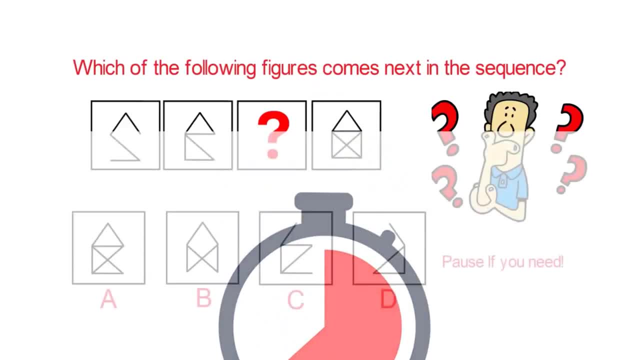 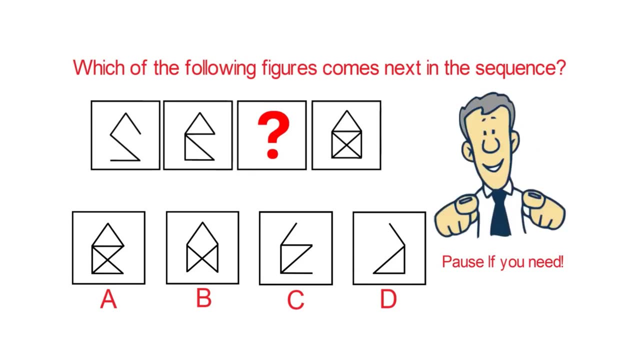 to 30 seconds. This is about as much time as you get on the test. You can pause this video to see if you can come up with the solution. Did you make your choice. Let's go ahead and continue so we can get to the correct solution together. 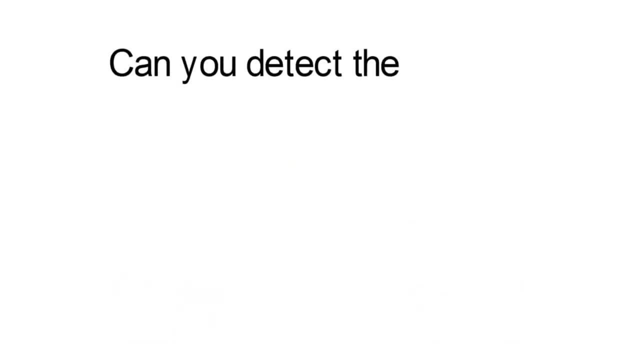 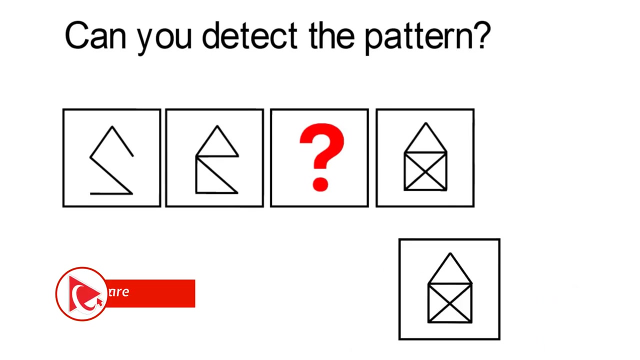 As you might have figured it out by now, the key to solving this challenge is to understanding what exactly is happening here in these pictures, And the answer is that we're drawing the miniature house using straight line And, the most important point, that we're tracing this house continuously until the house is. 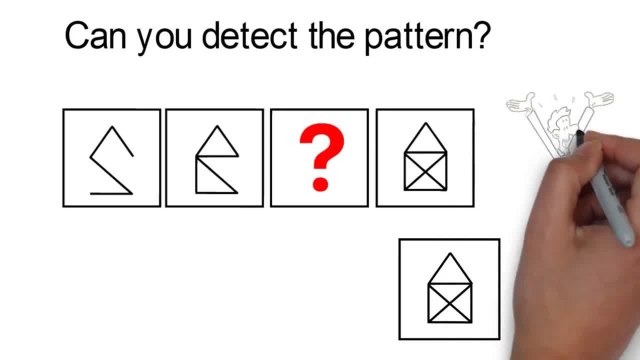 built. Once you understand this part of the problem, it's time to start the next step. Once you understand this part of the problem, it's time to start the next step. It's easy to solve. Let's draw this house step by step. There are eight lines in. 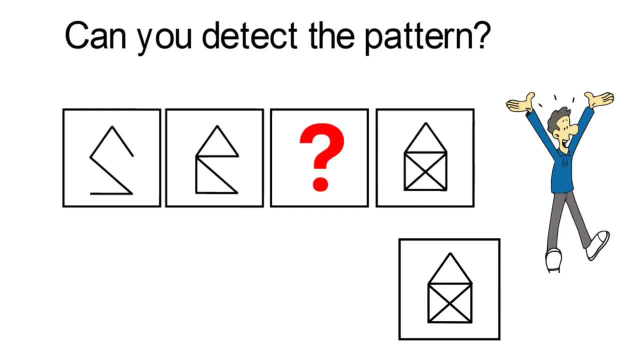 the final house. Let's draw all eight lines one by one: One, two, three, four, five, six, seven and eight. Now, having this information handy, we can go back to the original problem and easily see the solution, And the correct answer here is choice A. 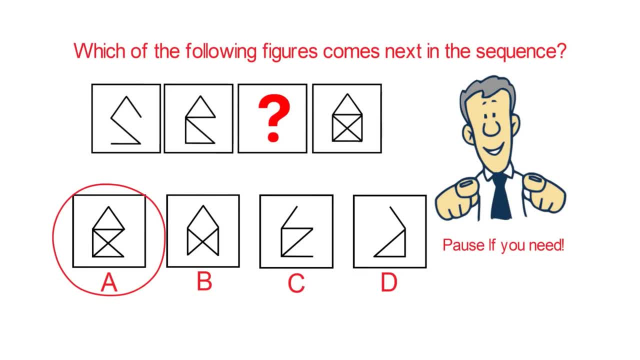 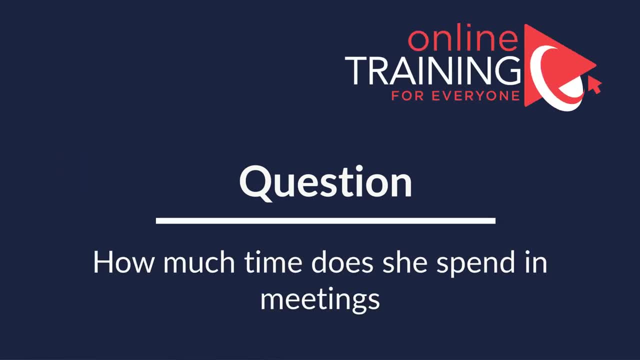 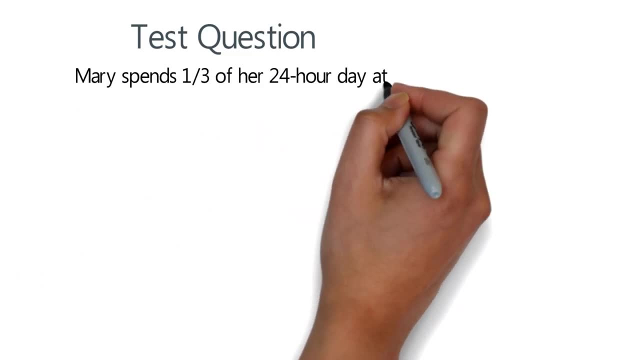 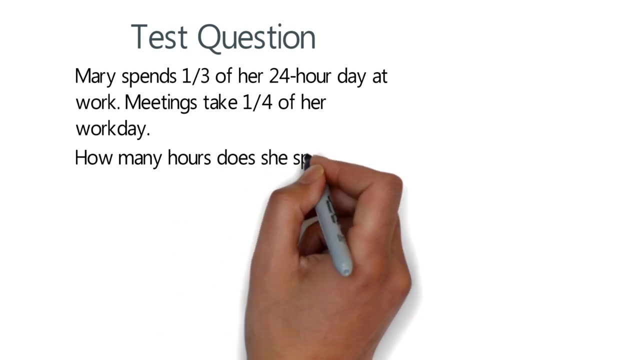 Hopefully you've nailed this question and now know how to answer similar problems on the test. Here's an interesting question which validates how well you do planning of your day-to-day work. Mary spends one-third of her 24-hour day at work. Meetings take one-fourth of her workday. How many hours does she spend in? 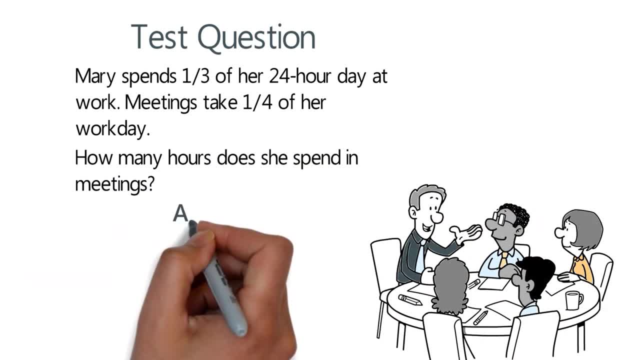 meetings. You have four different choices: Choice A- One hour and thirty minutes. Choice B- Two hours. Choice C- Two hours and thirty minutes. And choice D- Three hours. Give yourself 10 to 15 seconds, maybe a bit longer. 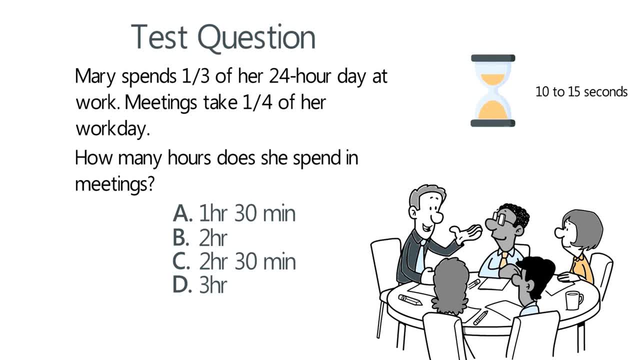 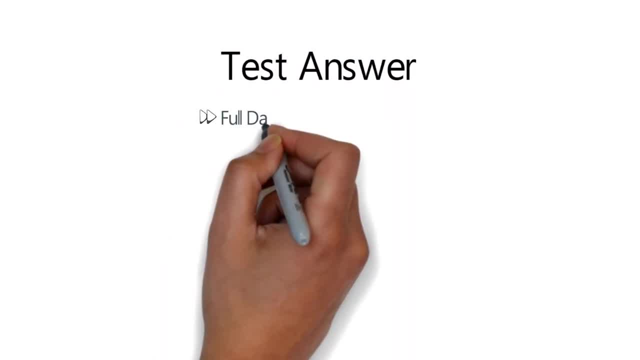 depending how well you typically solve these types of problems. Ready or not, let's go ahead and solve this challenge together. As you might be well aware, full day has 24 hours. Mary's working hours are very typical. They represent one-third of the full day, which is 8 hours, And we calculate it by multiplying. 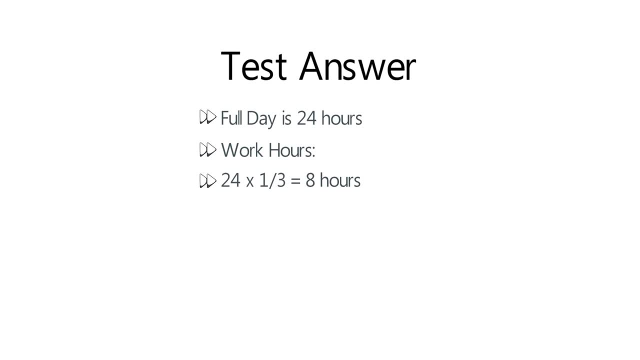 24 by one-third, or actually dividing 24 by three. Meetings take one-fourth of her workday. So to calculate how much time she spends in meetings, we need to multiply 8 hours by one-fourth And the result is 2 hours. So the correct answer is choice B, Two hours. Hopefully you've. 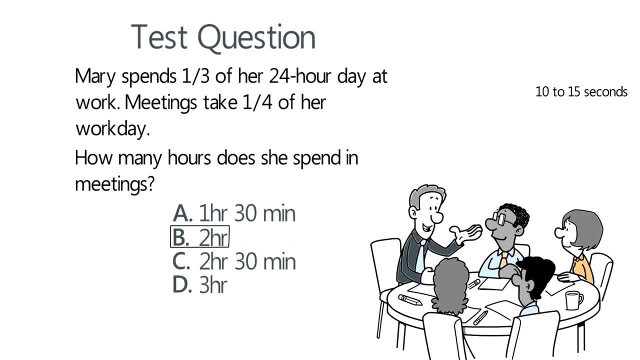 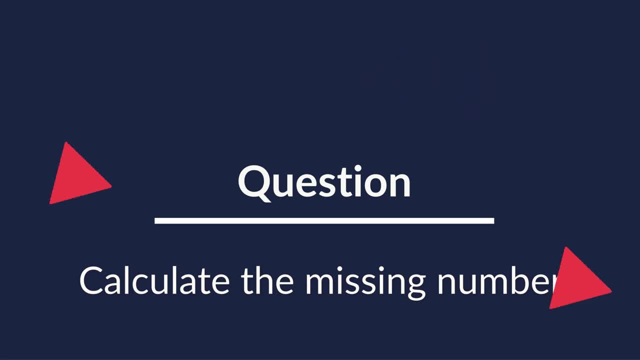 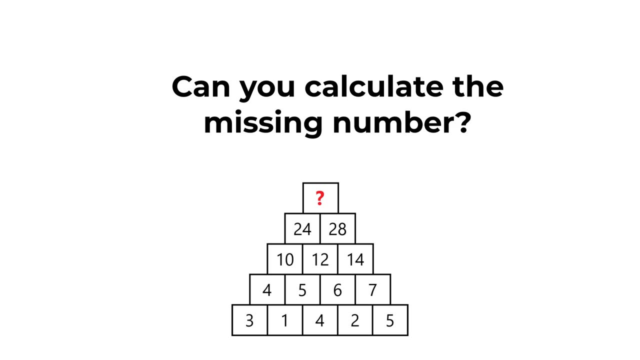 nailed this question. We now know how to answer similar problems in the test. Here's one of my favorite questions, and it is my favorite because it is so unusual. You are presented with the pyramid. Pyramid contains five different layers. If we go from the top to bottom, you have a question mark. 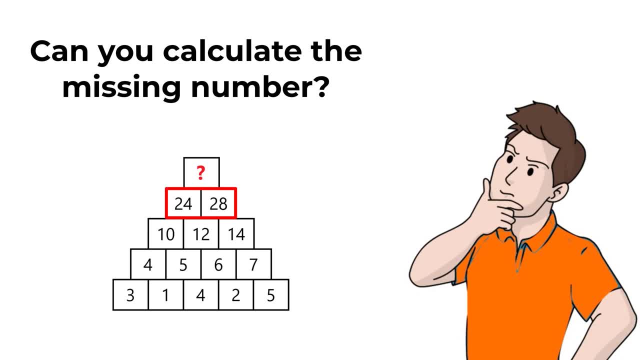 This is the number that you need to uncover. The next layer contains numbers 24 and 28.. Number below this contains numbers 10,, 12, and 14.. Next layer has 4,, 5,, 6, and 7.. 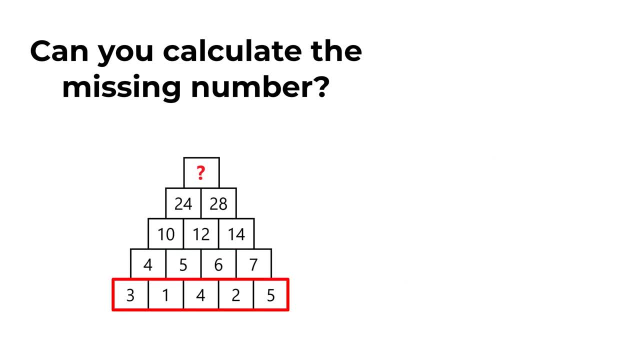 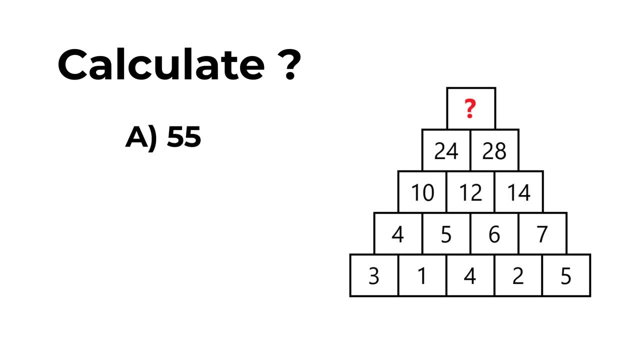 And the last layer has numbers 3,, 1,, 4,, 2, and 5.. You are presented with four different choices for the missing number: Choice A: 55.. Choice B: 56.. Choice C: 57.. 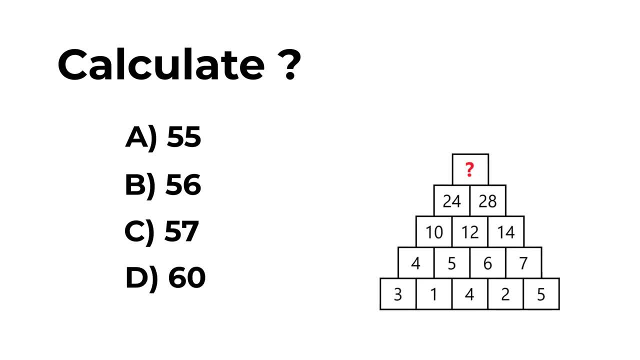 And choice D: 60.. Do you see the answer? You will be surprised how simple it is to get to the answer When we go to the next step. give yourself 5,, 10, maybe 15 seconds to see if you can calculate. 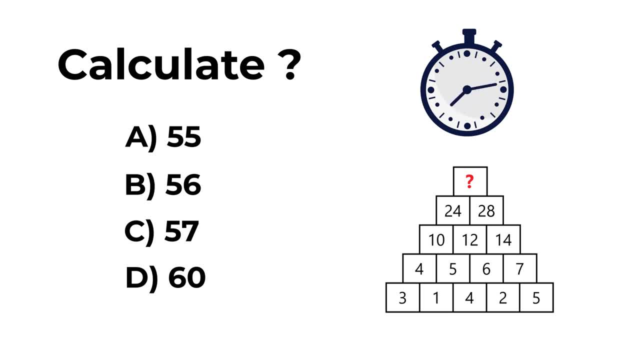 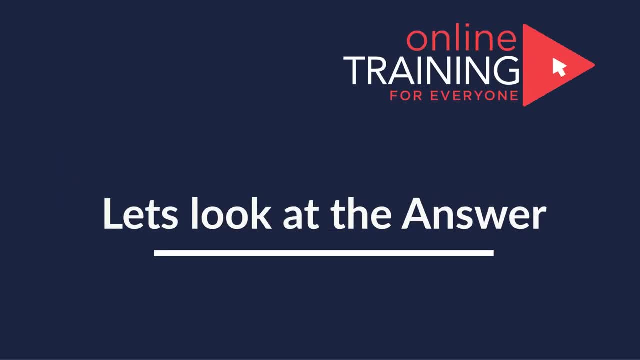 and get to the correct answer. Did you figure it out? Let's continue and see how we can get to the correct solution together. Well, here, to be honest, I tried to trick you. I went in describing numbers from top to bottom. 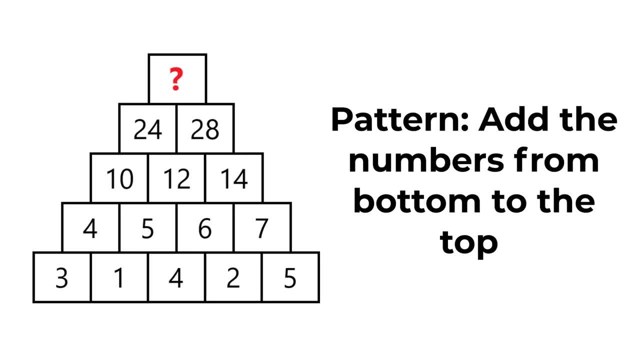 But in reality you should be looking at the numbers from bottom to the top. If we start from the bottom row, for example, with numbers 3 and 1, you see that the sum of 3 and 1 is 1.. 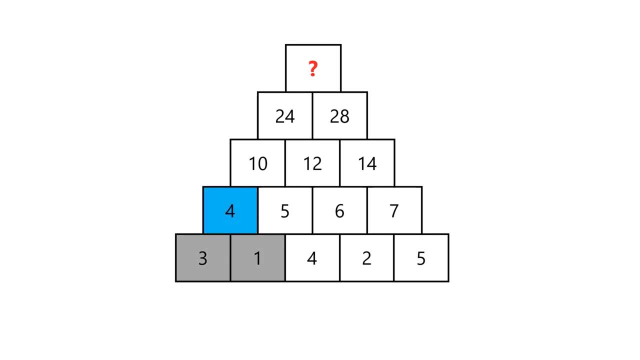 We'll add up to 4.. But then it gets trickier. If we go from the second row to the third row, you see that the 4 and 5 does not necessarily add up in 10.. 4 and 5 adds up in 9, and then you need to increment it by 1.. 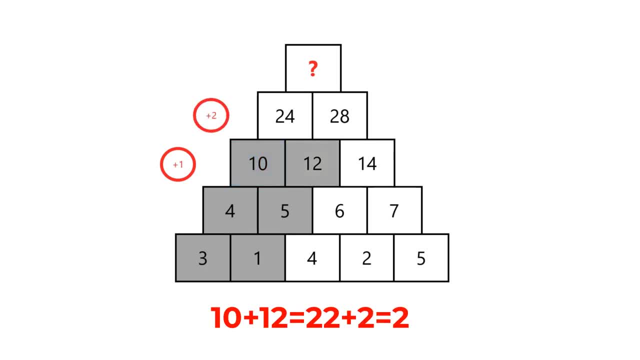 If you go to the next layer, you need to increment it by 2.. And then, in the final row, you need to increment it by 3.. So the correct answer here is choice 55.. Let's recap, Starting with the bottom row. 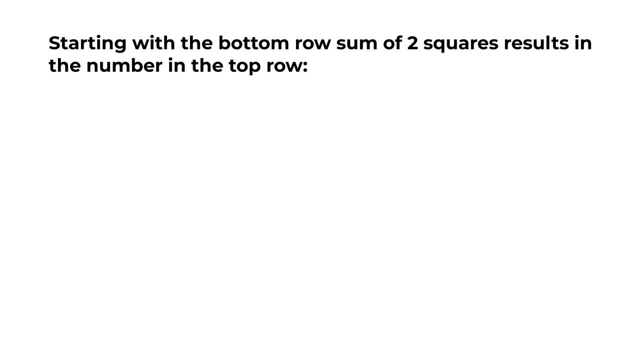 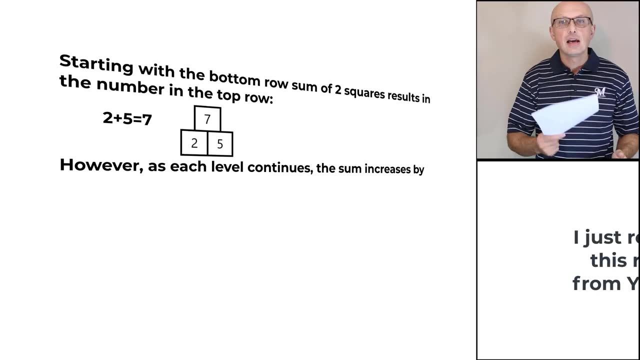 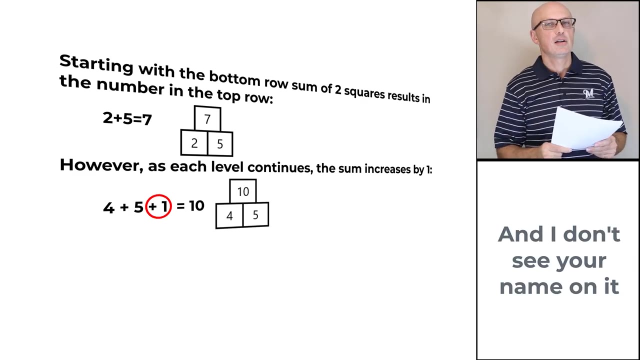 The sum of 2 squares results in a number in the next row. For example, 2 plus 5 equals 7.. However, as each level continues, the sum increases by 1.. For example, 4 plus 5, we need to increment and add 1 to get to 10..